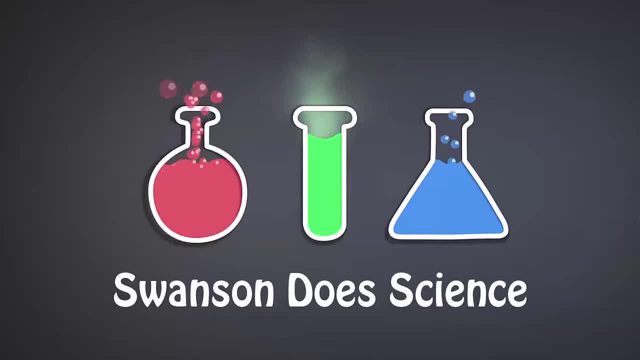 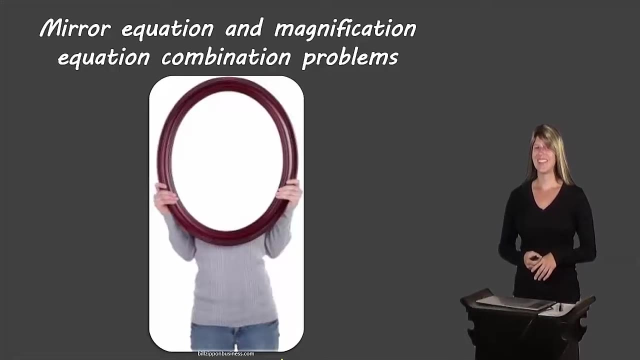 Hello students, Ms Swanson, here and today we're going to take a look at how to solve problems that use both the mirror equation and the magnification equation for mirrors. If you haven't yet watched the video on the mirror equation or the magnification equation, 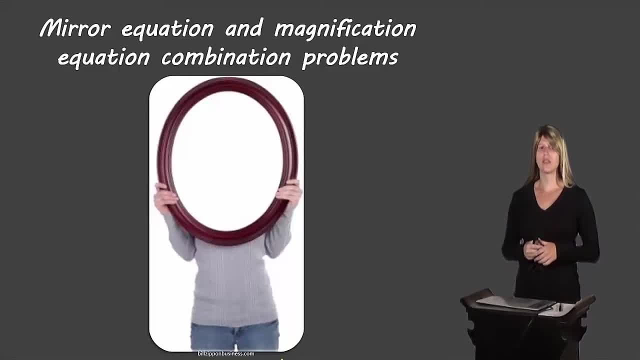 for mirrors. please watch those videos first. I'll put a link in the description box below, because you'll need to know that information in order to understand the lesson that we're doing today. So we have one learning goal here: to calculate magnification. object height. 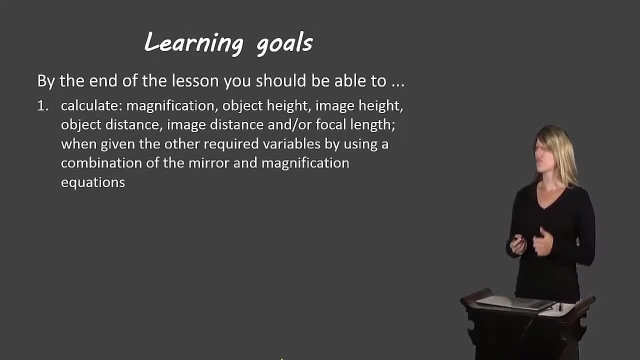 image height, object distance, image distance or focal length when given the other required variables using a combination of the mirror equation and the magnification equation. So let's just do a little bit of a review here. This is our mirror equation, and in white. 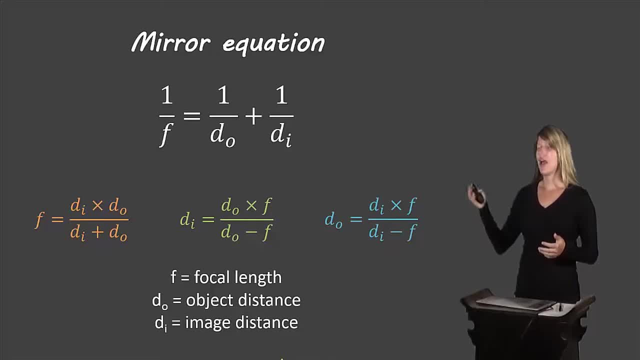 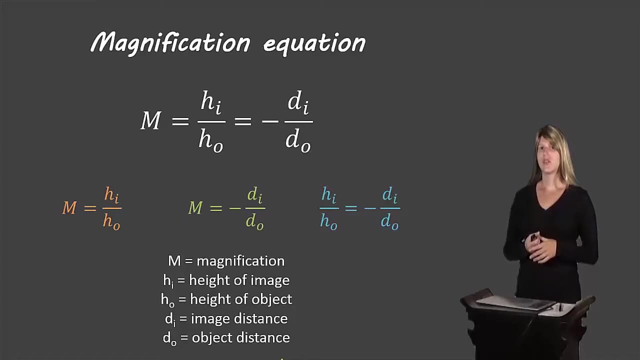 it shows the original formula for the mirror equation. and then the equations below show the different versions of the equation where each of the individual variables are isolated, so that we could actually use those equations to solve problems. And then here's our magnification equation, Again in white. it shows the full form of the equation, and in white it shows: 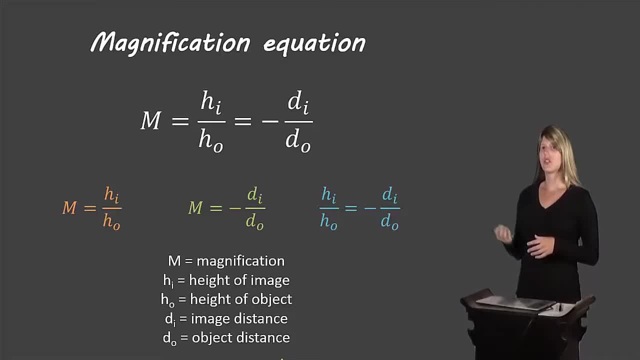 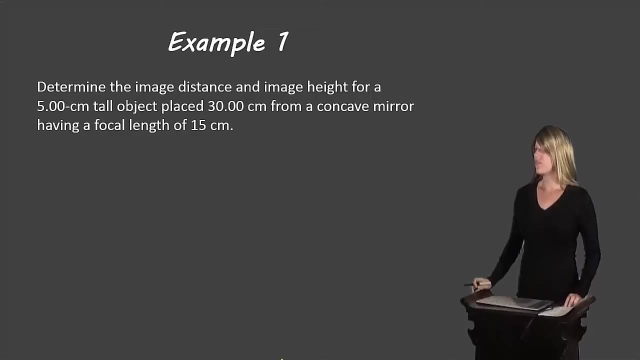 the full format of the magnification equation, and then the orange, green and blue equations show the different pieces of the magnification equation that can be used in isolation. So let's take a look at an example here. Determine the image distance and image height for a five. 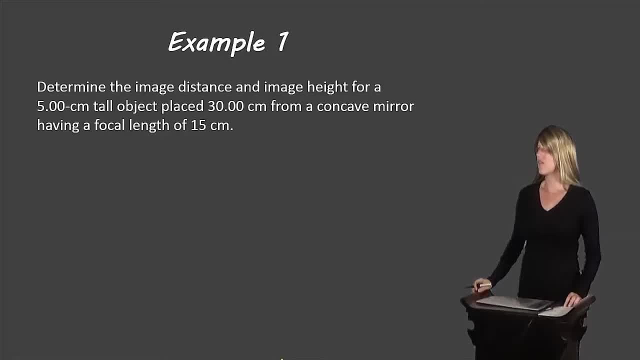 centimeter tall object placed 30 centimeters from a concave mirror having a focal length of 15 centimeters. So let's find the information that we have in the question. So we have a five-centimeter tall object placed 30 centimeters from a concave mirror having a focal length. 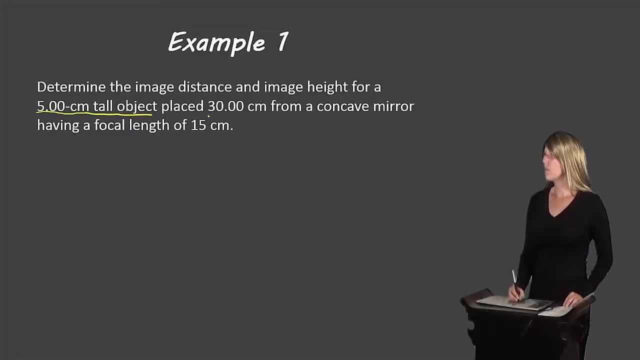 5.00cm tall object, placed 30.00cm from a concave mirror that has a focal length of 15cm. So let's write out our given information. So we have a 5.00cm tall object. so that's the height of the object, which is 5.00cm. 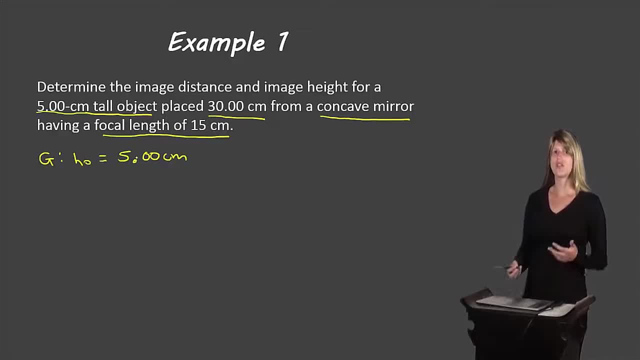 And I chose positive 5.00 because HO is always a positive number. And then that object is placed 30.00cm from a concave mirror. Now I chose positive 30.00 because DO is always a positive value. And then we have a focal length of 15cm. 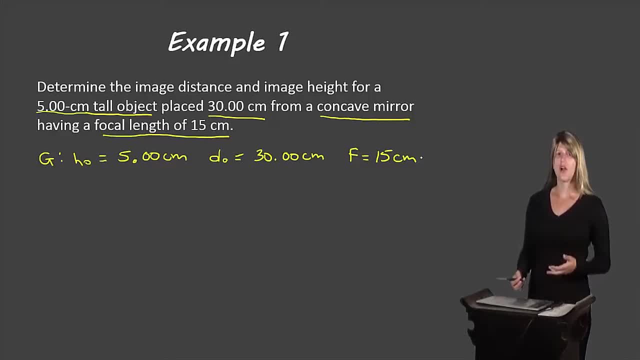 I chose positive 15 for this because it tells us it is a concave mirror And concave mirrors have the convention of a positive sign. So what is required? We need to find the image distance, which is DI, and the image height, which is HI. 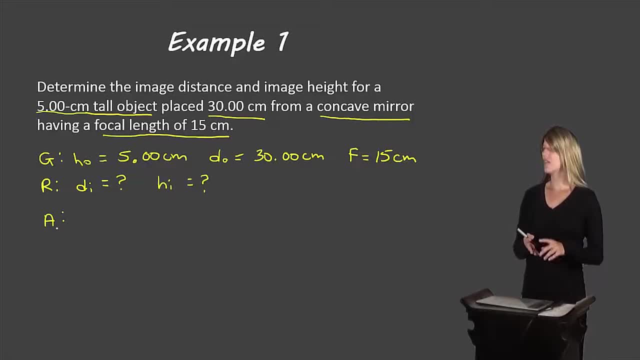 So what can we do to solve this problem? We have information about heights, distances and focal length. If we tried using the magnification equation, we don't have enough information to be able to use any of those pieces of the equation. However, 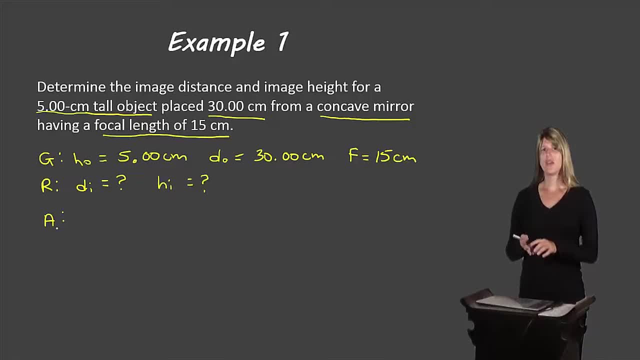 With DO and with F we can find DI using the mirror equation. So with the distance of the object and the focus we can use the mirror equation. So let's do that now. So for our analysis we'll use 1 over F, equals 1 over DO plus 1 over DI. 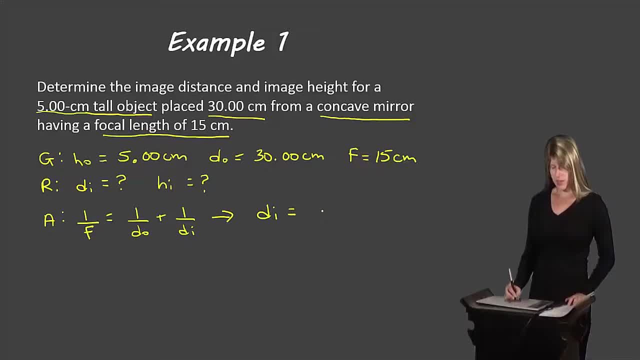 And we can rearrange that equation So that DI is equal to DO times HI, DI times F over DO minus F, And so this here is all part A. So if we substitute and solve here, DI is going to equal 30.00cm times 15cm over 30.00cm. 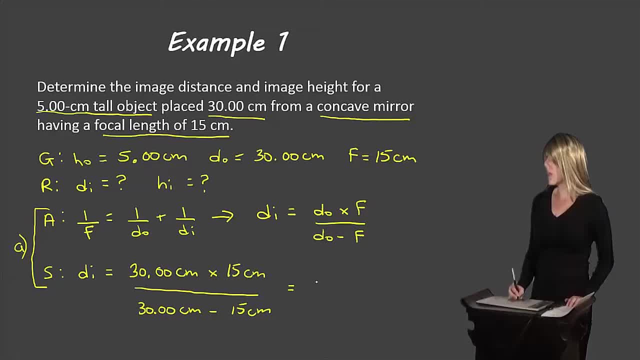 minus 15cm. So if we do that math we'll end up with 30cm. Only two significant digits here, because 15 only has two significant digits. So I'm going to switch to the next slide. We'll lose this information here, but you should have it copied on your page already. 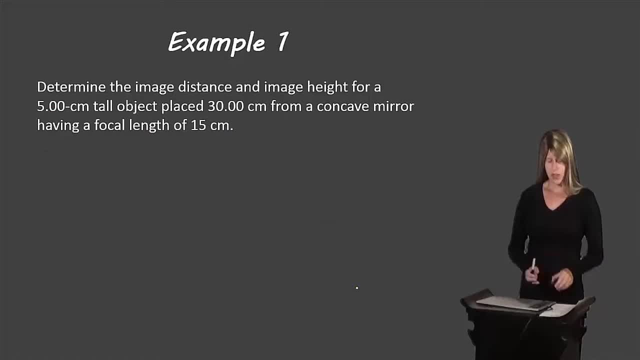 so that you can refer back to these values. So now we're going to do the second part, So we have more information so that we can now use the magnification equation. If we use this version of the magnification equation, HI over HO equals negative DI over. 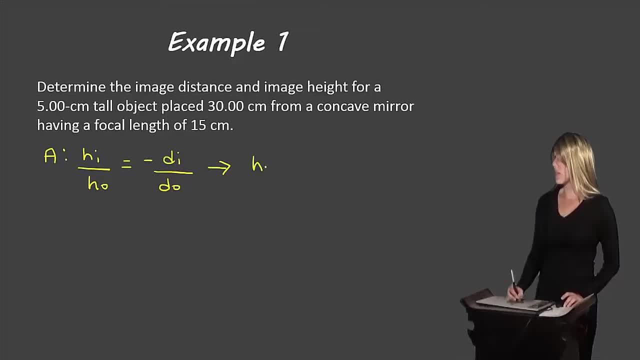 DO. we can rearrange that equation so that HI is equal to negative DI times HO over DO. So this all is part B. So this all is part B. So we're able to use this equation now because we solved for DI, Now for part A. 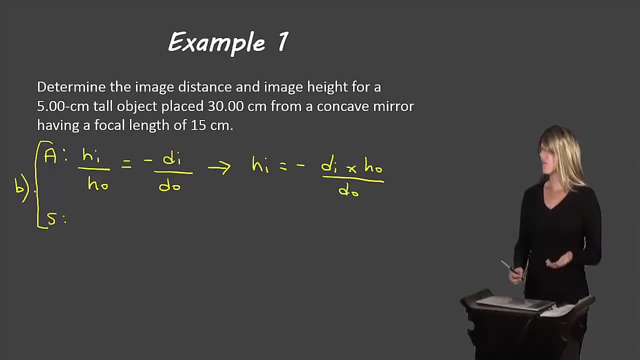 So we're able to use this equation now because we solved for DO i, we already had d? o and we already had h o. so now if we substitute and solve, we have negative and our d i that we just solved is 30 centimeters times our h? o, which was 5.00 centimeters. 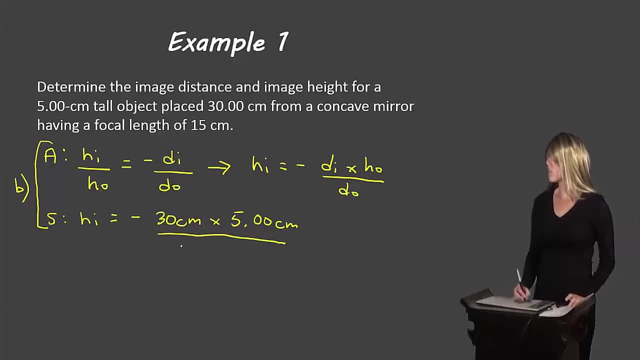 over our d? o, which was 30.00 centimeters. and if we solve that math there we end up with negative 5.0 centimeters- again two significant digits so we can write our sentence here. so the inverted real image. so how did i know that it was inverted? 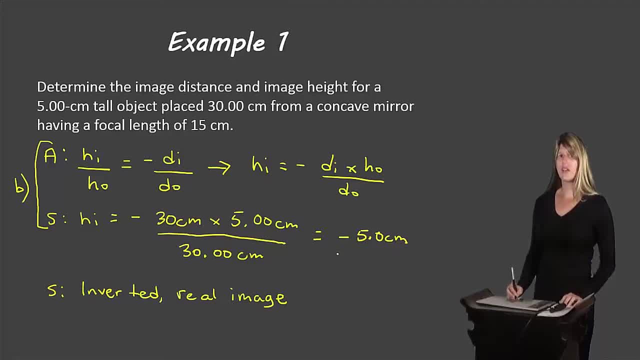 and real well, our h? i is a negative value, which means it's an inverted image, and we know that it's real because d? i, from our part, a, was a positive value and d? i is positive for real images. so our inverted real image is 5.0 centimeters tall and 30 centimeters from. 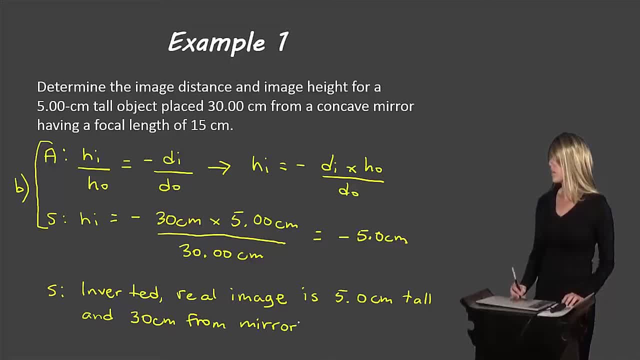 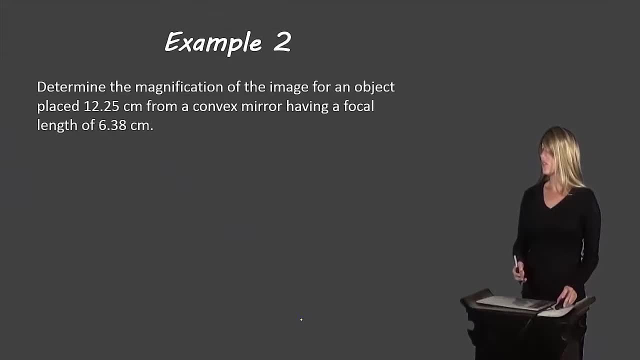 the mirror. so this is how we would solve a problem like that. let's take a look at another type of example. determine the magnification of the image for an object, place 12.25 centimeters from a convex mirror having a focal length of 6.38 centimeters. so again, we're given lots of. 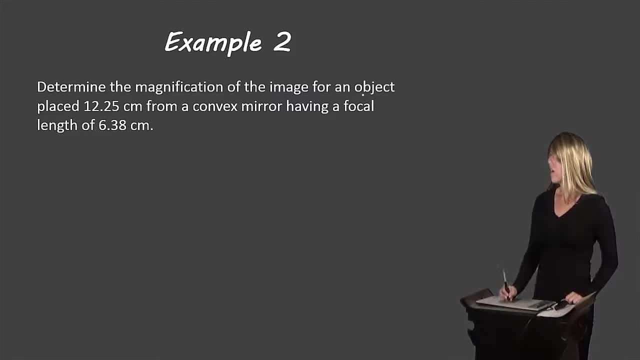 information, so let's find all of it. so we have an object place 12.25 centimeters from a convex mirror that has a focal length of 6.38 centimeters. so let's write down our given information. so the original object is placed this far from the mirror. so that will be d? o, the distance of the object is. 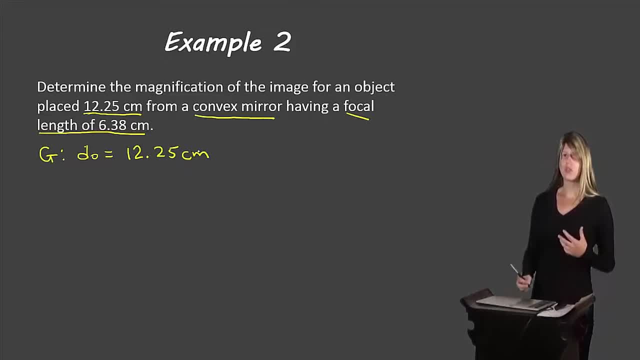 12.25 centimeters. i chose positive 12.25 because d? o is always a positive number. and then we have the focal length of 6.5 centimeters and then we have the distance of the object, which is 12.25 centimeters. so we need to write down the magnification of our object, that we're meant to. 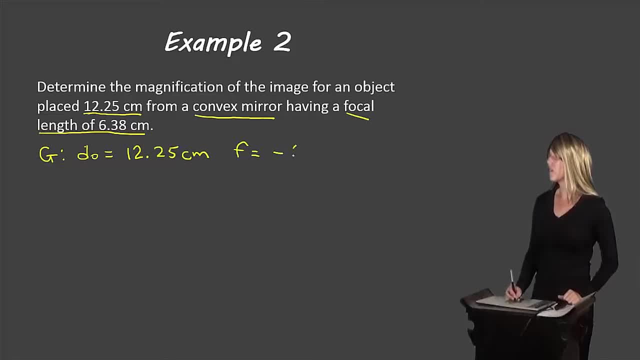 write. so let's just go ahead and look at this object there and we're just going to write negative 6.38 centimeters. now it tells us we're dealing with a convex mirror, which means we need to write negative 6.38 centimeters. so what is required of us? we need to find the magnification. 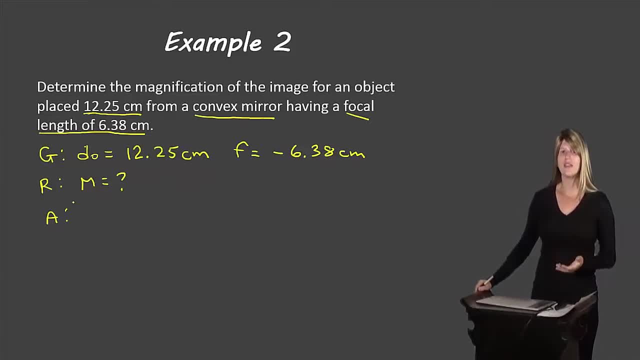 so how do we analyze this question? well, in order to find magnification, we could use d? o, but we would also need to know what d? i is, and we don't have any information about d? i right now. however, we can. However, because we have DO and we also have the focal length, we can calculate DI and 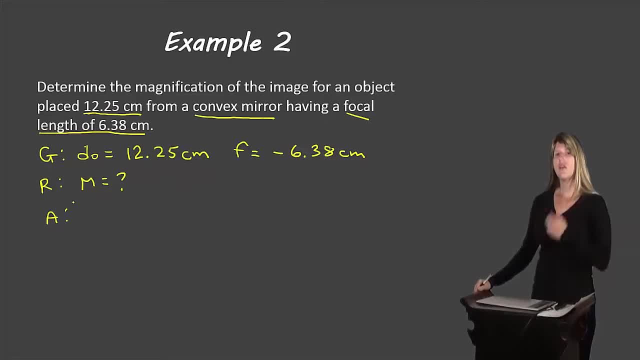 then using DI and DO from the question, we can then solve for the magnification. So that's what we'll do here. So we'll start off by using our mirror equation. So 1 over F equals 1 over DO, plus 1 over DI, and we can rearrange this equation for DI. 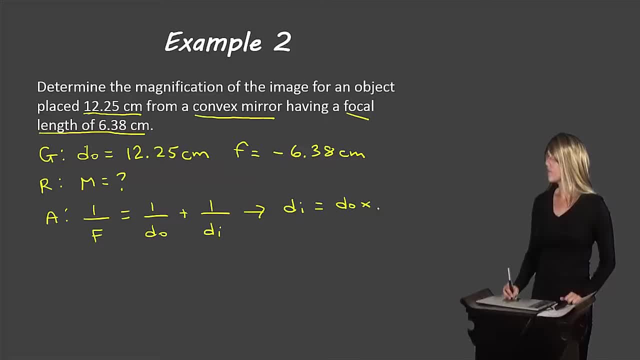 so that will equal DO times F over DO minus F, And so this all here is the first part, part A. So to substitute and solve here we'll have DI equals, and DO is 12.25 cm times negative 6.38 cm. 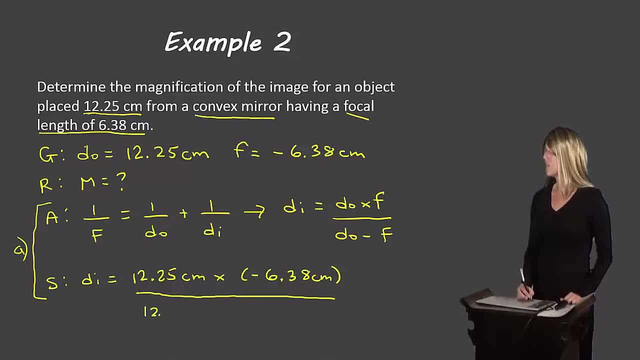 Over and then DO 12.25 cm minus negative 6.38 cm, And that will give us a final answer of negative 4.20 cm. So now we have DI, we can use that information to calculate the magnification. 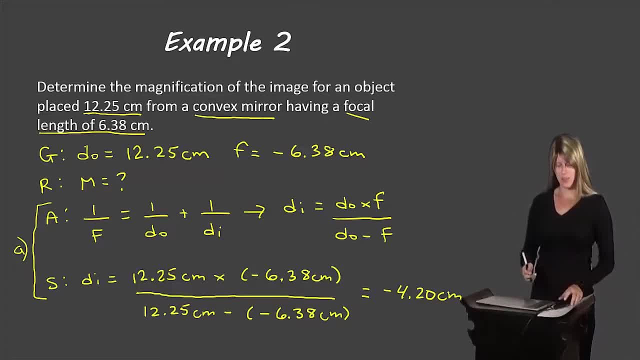 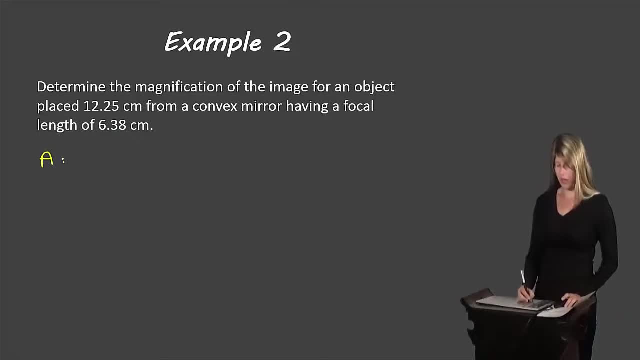 So, again, you should write all this down. When I switch slides, you won't have this information anymore up here. So for part B, we can now use our magnification equation and we'll use the piece that deals with distances and magnification.